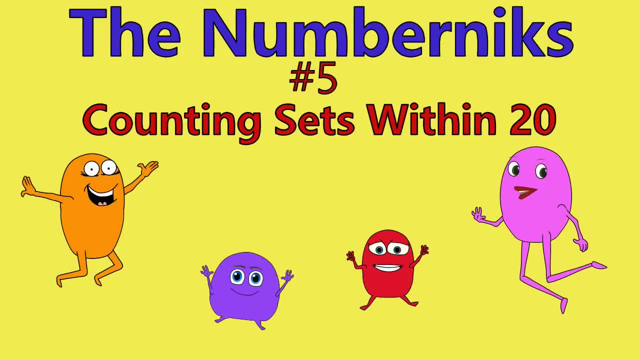 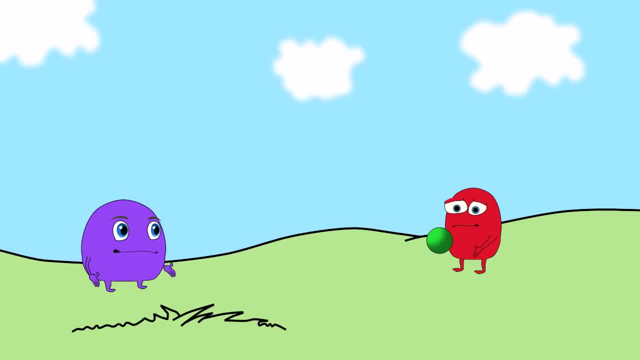 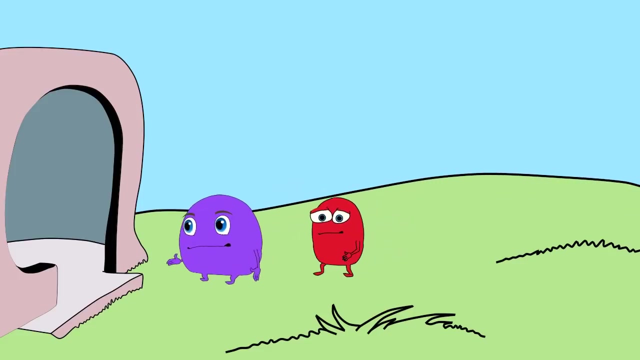 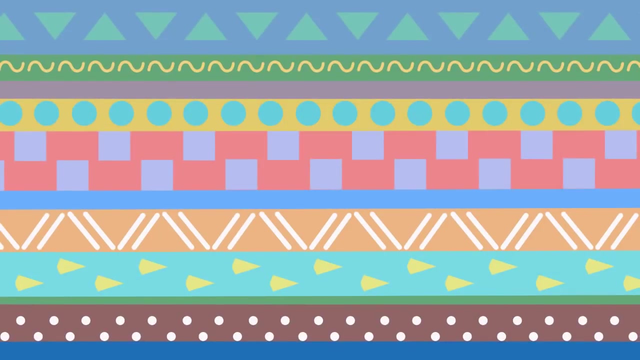 That was fun. What should we play now? I know Let's go to the math game dimension. Good idea, Now that we know how to count to 20, it's going to be so much fun. Woo, Bring on the counting. I know how Let's go. I know numbers now. 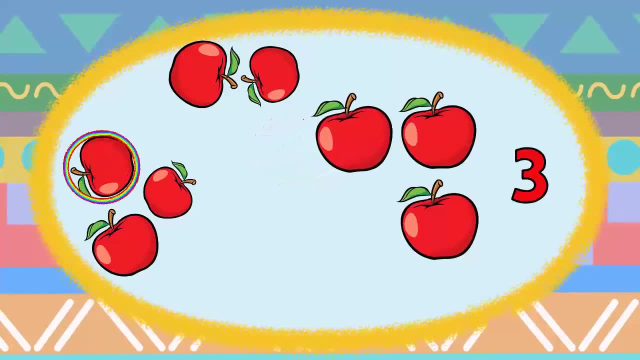 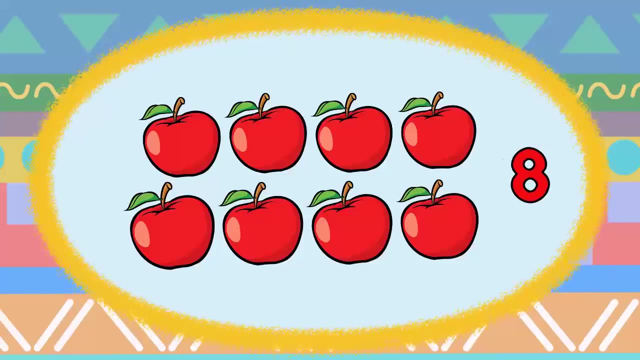 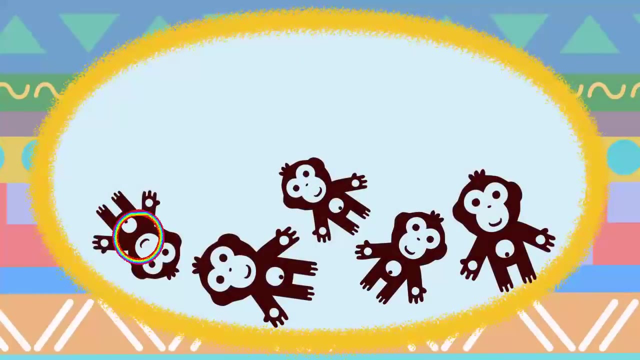 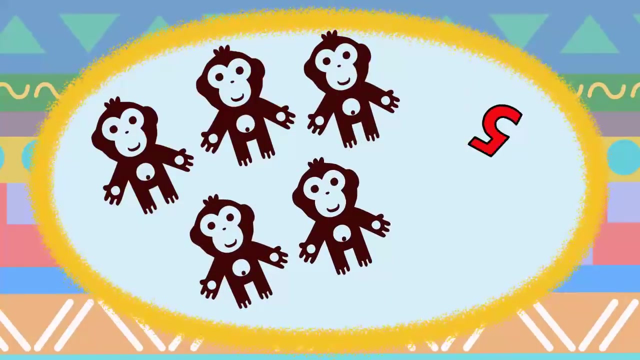 1,, 2,, 3,, 4,, 5,, 6,, 7, 8.. 8 apples Way to go: 1,, 2,, 3,, 4,, 5,, 5 monkeys. 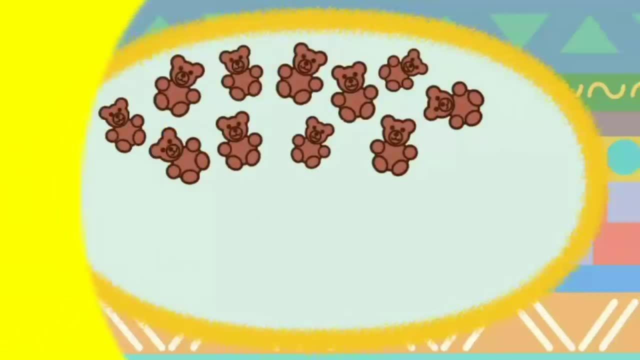 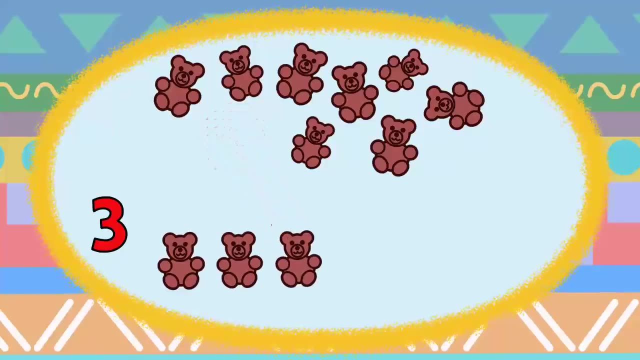 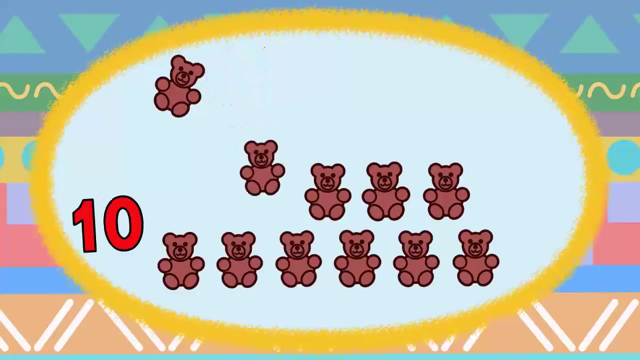 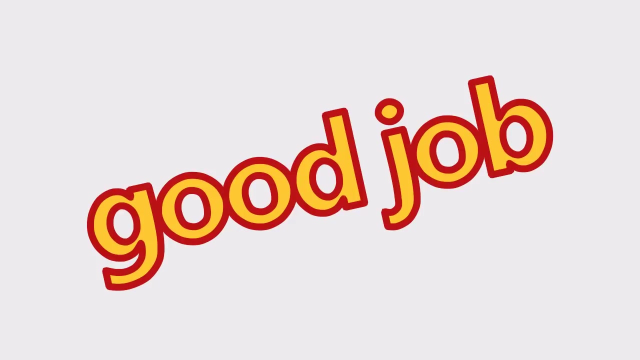 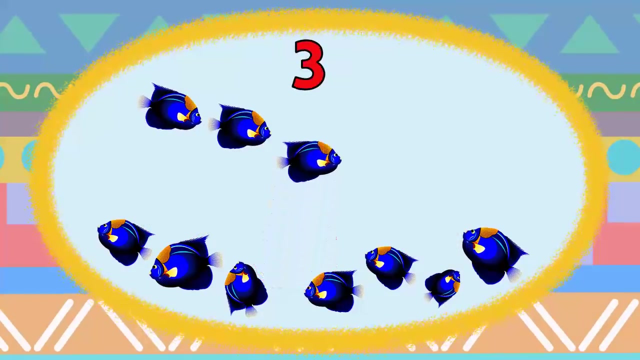 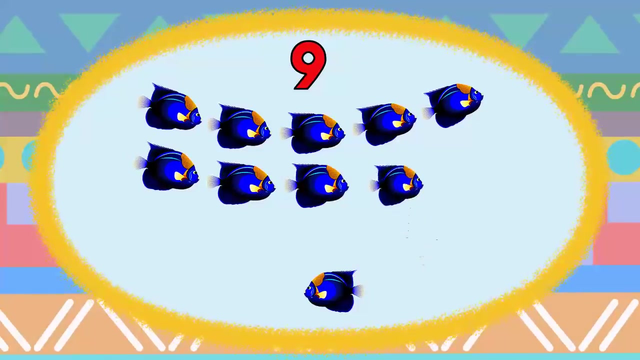 Awesome, Awesome. 1,, 2,, 3,, 4,, 5,, 6,, 7,, 8., 8,, 9,, 10,, 11.. 11 teddy bears: Good job. 1,, 2,, 3,, 4,, 5,, 6,, 7,, 8,, 9,, 10.. 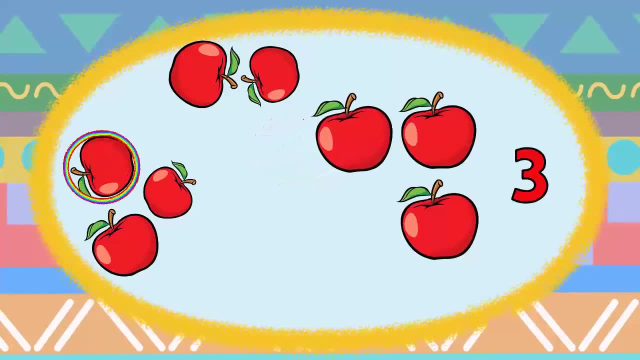 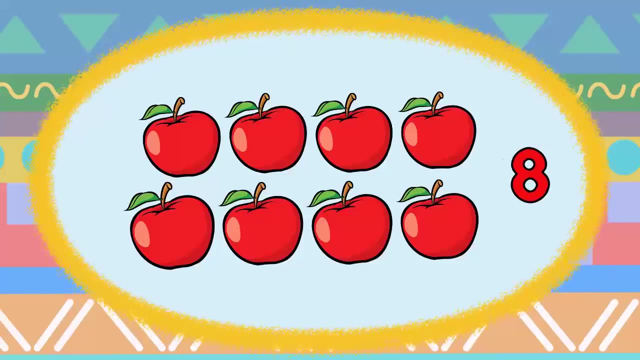 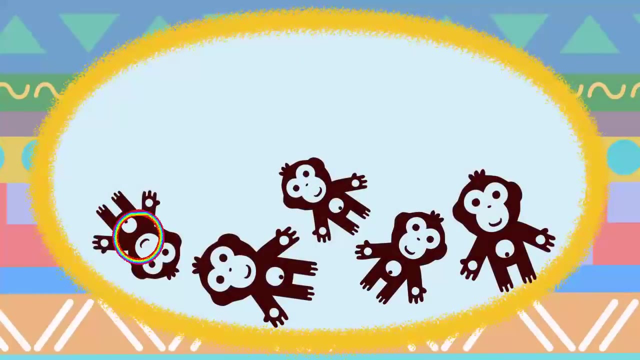 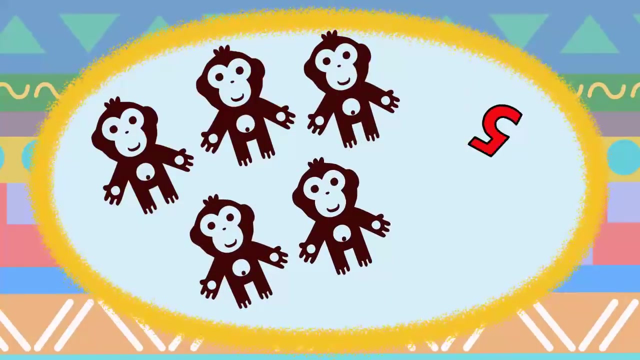 1,, 2,, 3,, 4,, 5,, 6,, 7, 8.. 8 apples Way to go: 1,, 2,, 3,, 4,, 5,, 5 monkeys. 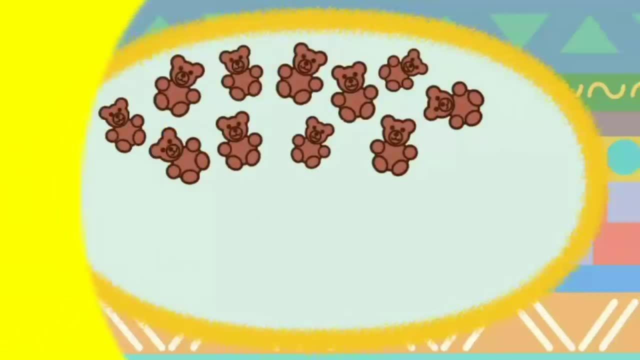 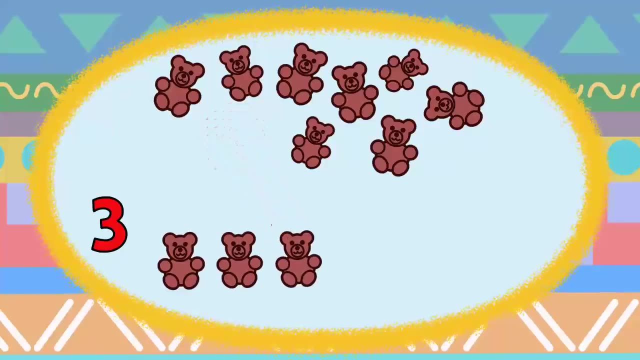 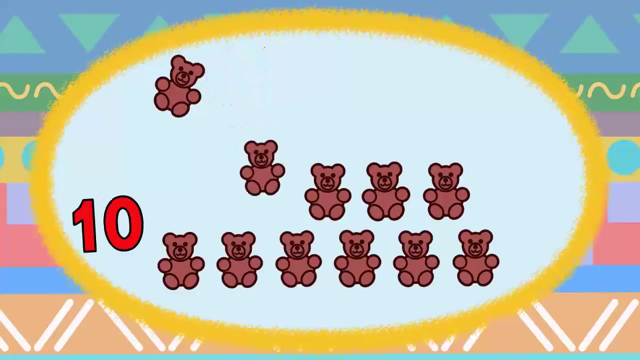 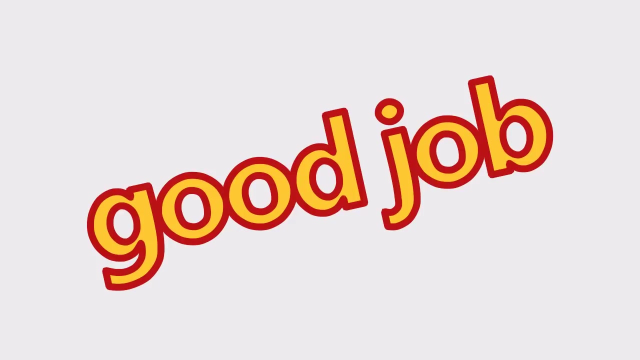 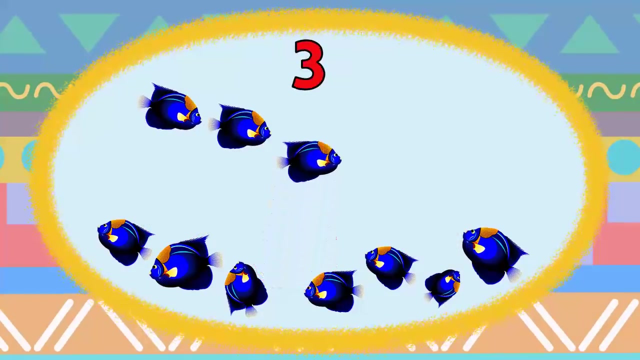 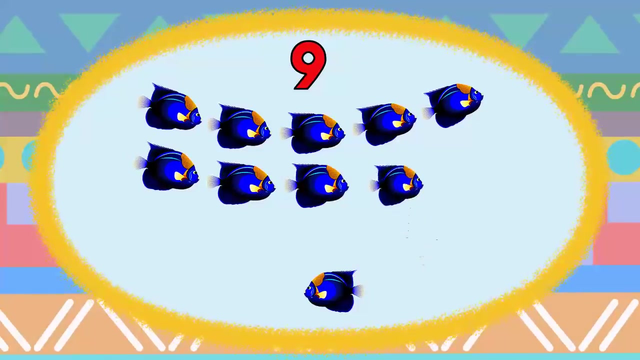 Awesome, Awesome. 1,, 2,, 3,, 4,, 5,, 6,, 7,, 8., 8,, 9,, 10,, 11.. 11 teddy bears: Good job. 1,, 2,, 3,, 4,, 5,, 6,, 7,, 8,, 9,, 10.. 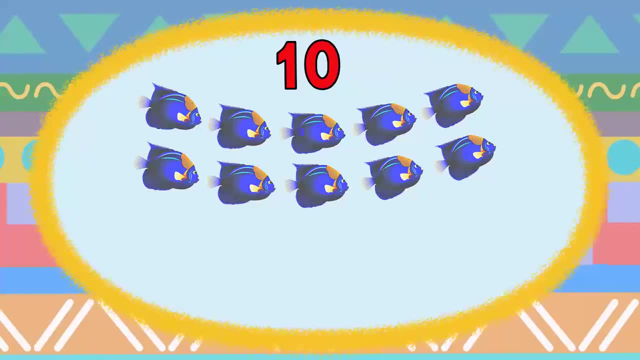 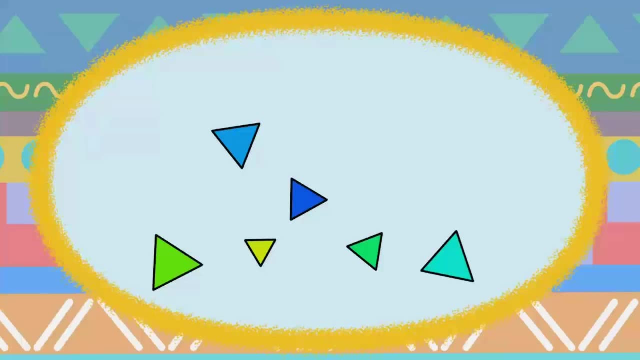 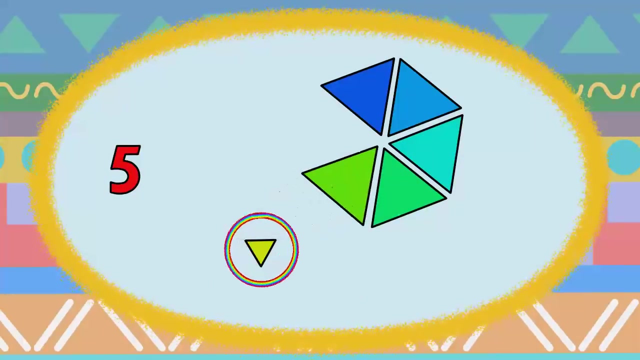 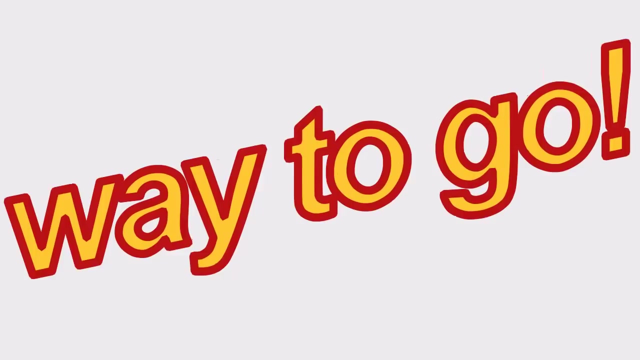 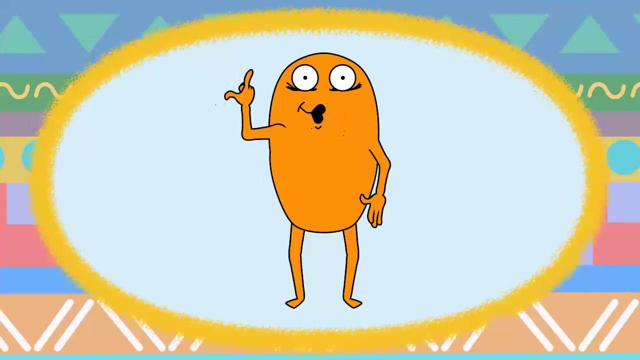 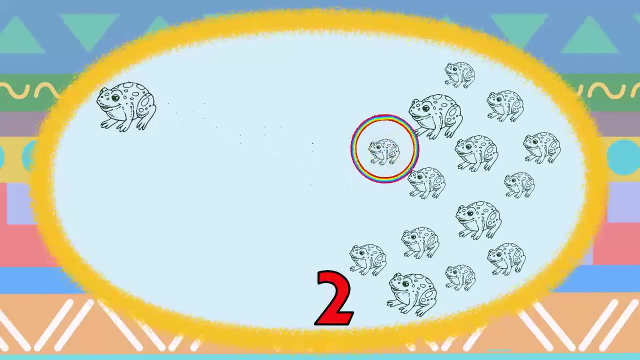 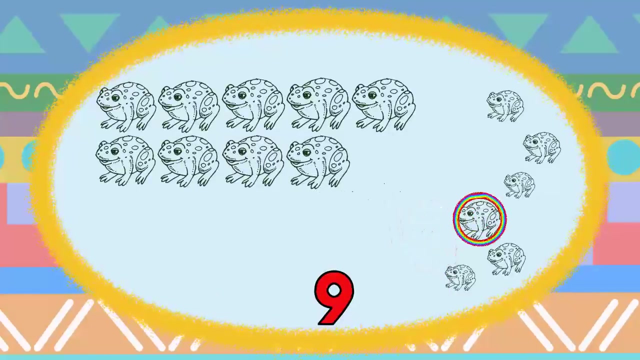 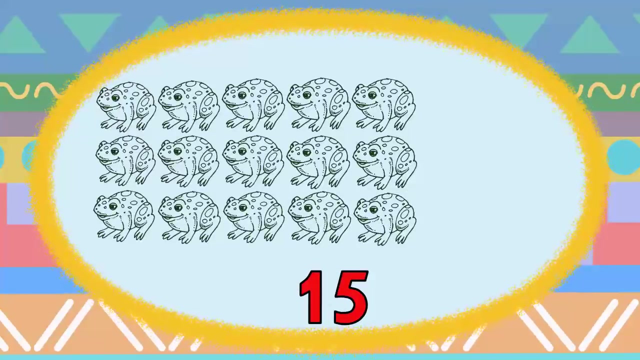 10 fish, All right. One, two, three, four, five, six, Six, triangles. Way to go, Way to go. Now it's your turn. kids. Count all the things you see. Fifteen frogs- Awesome. 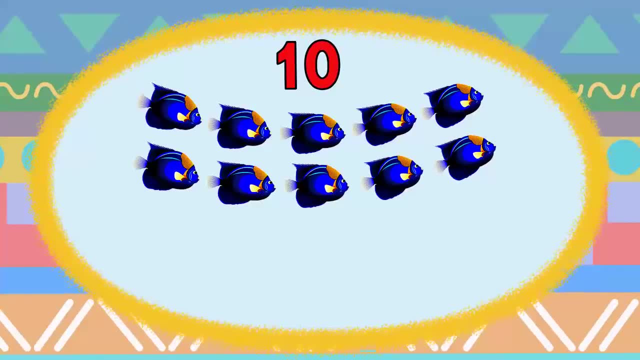 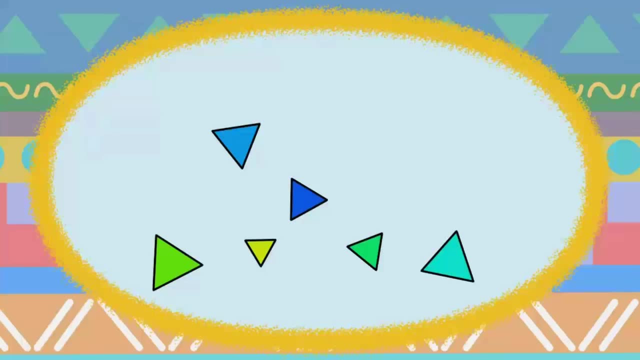 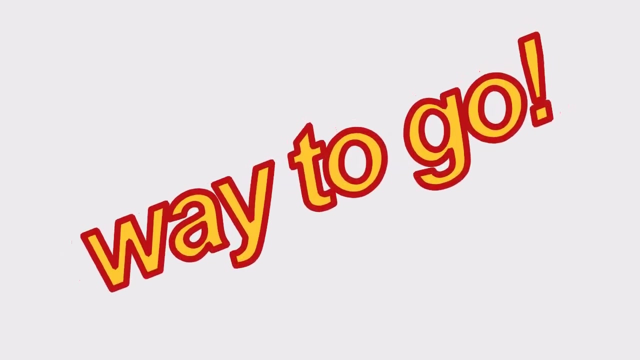 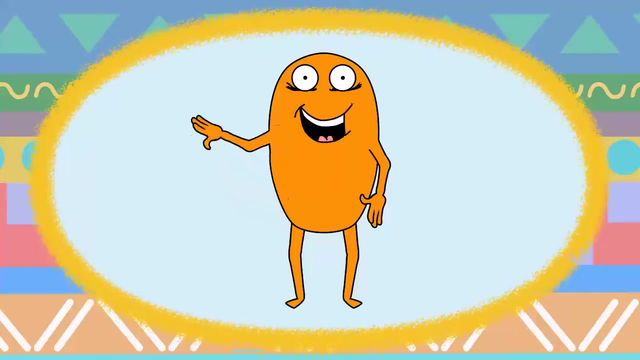 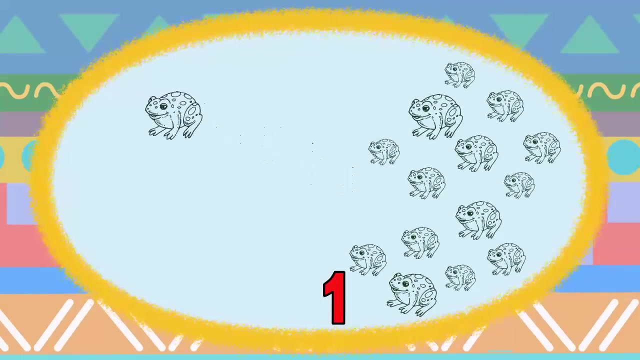 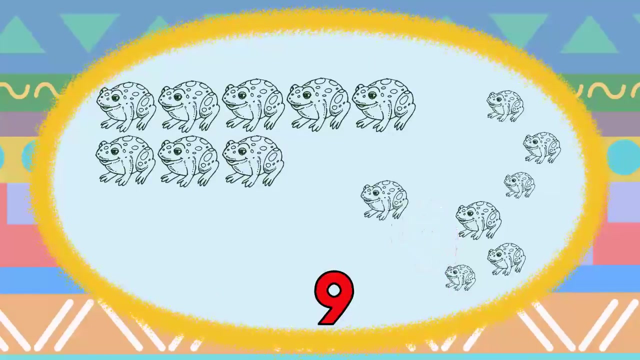 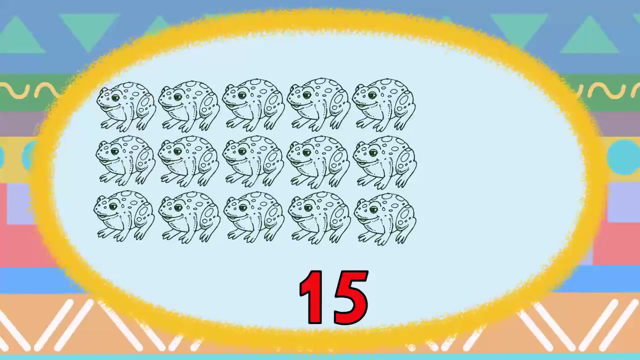 10 fish, All right. One, two, three, four, five, six, Six, triangles. Way to go, Way to go. Now it's your turn. kids. Count all the things you see. Fifteen frogs- Awesome. 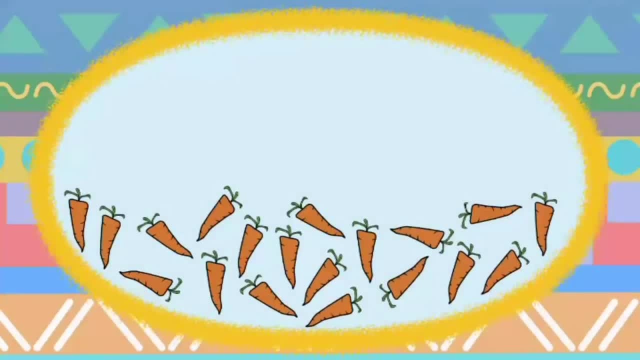 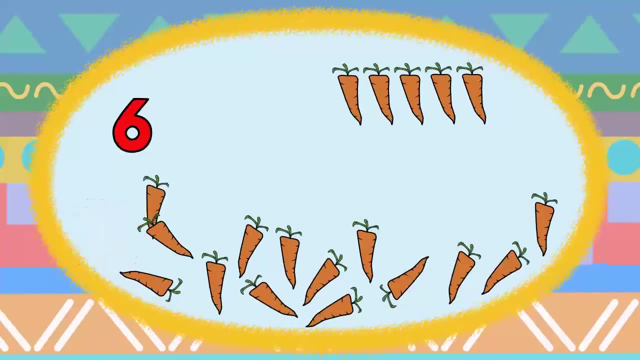 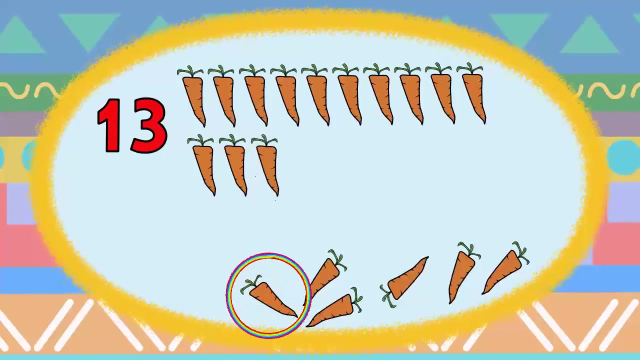 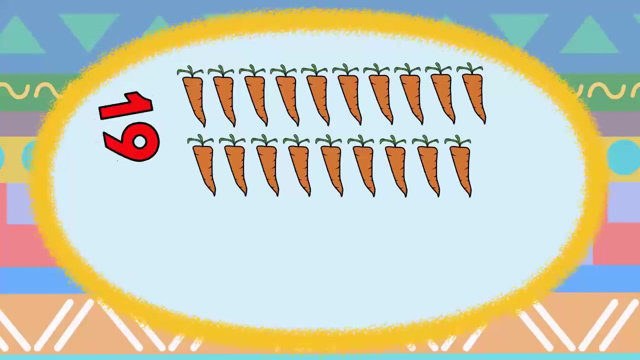 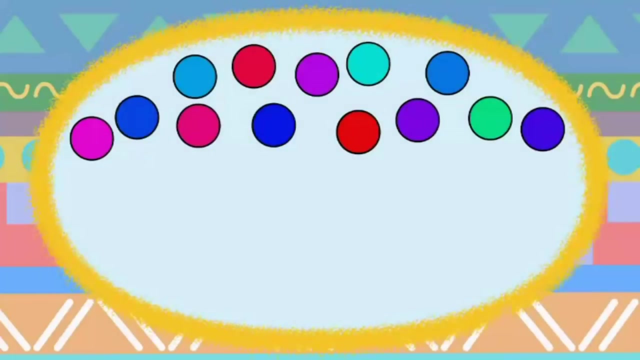 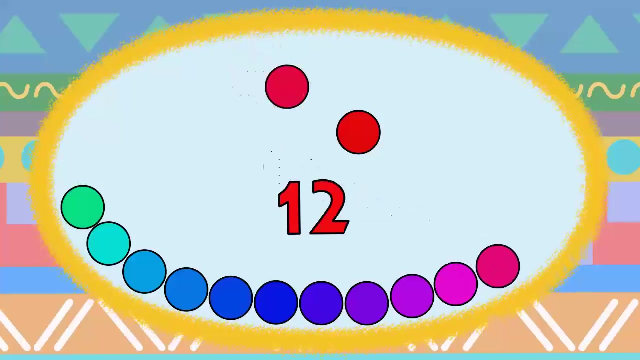 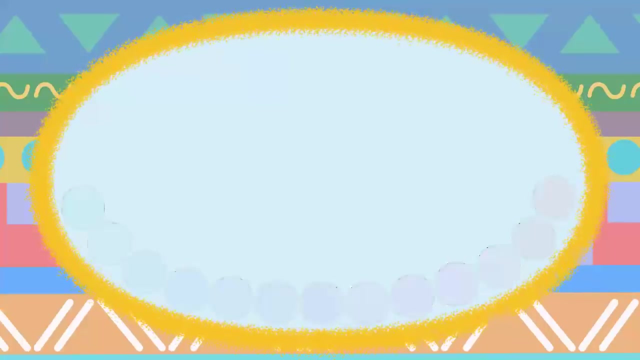 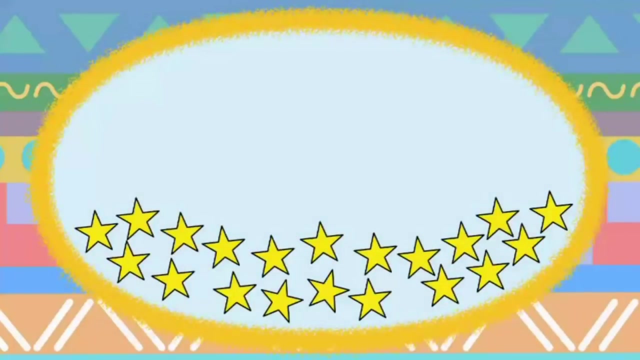 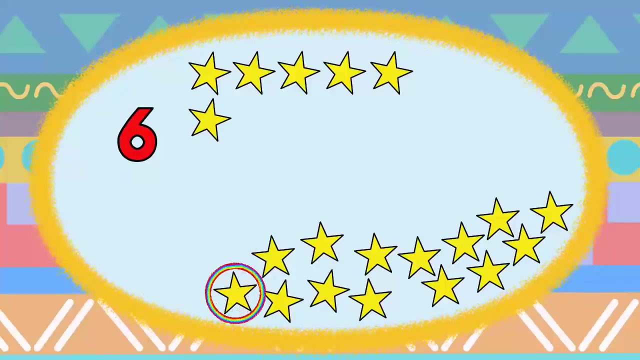 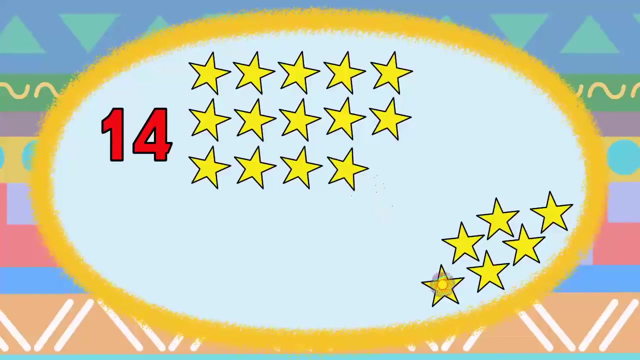 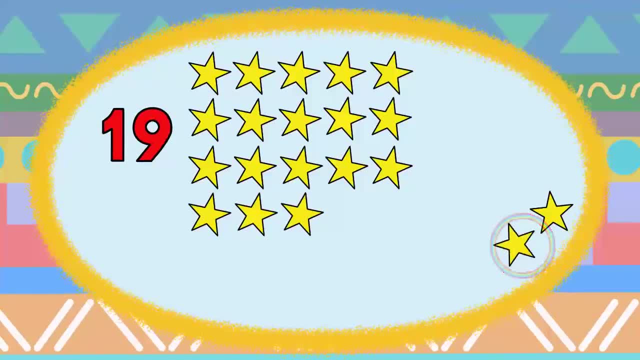 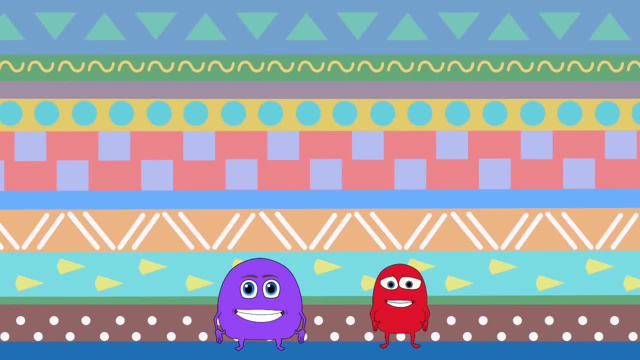 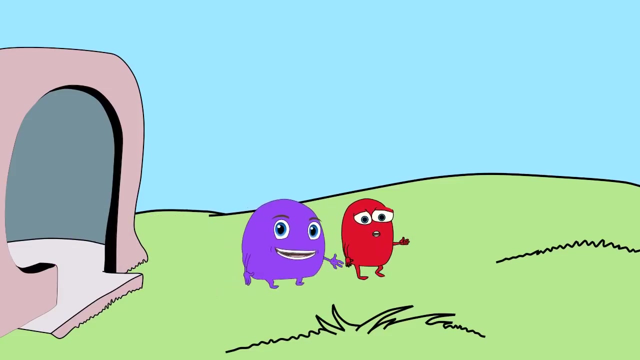 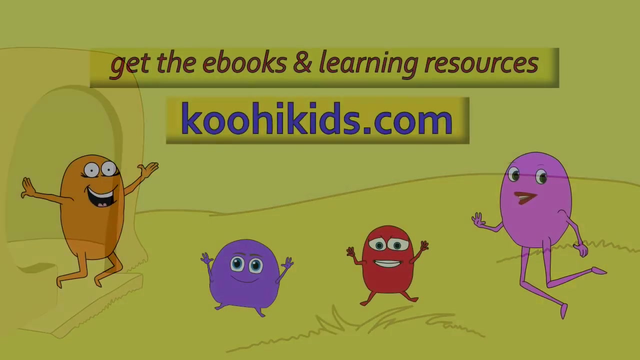